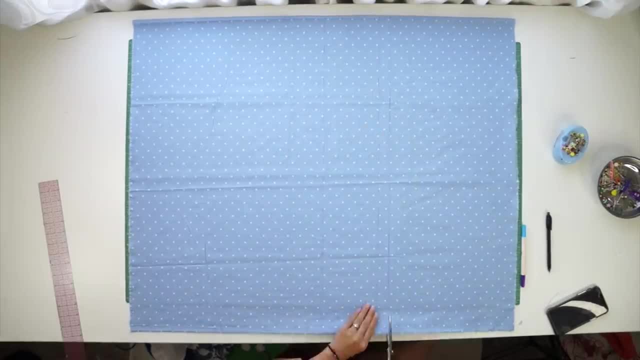 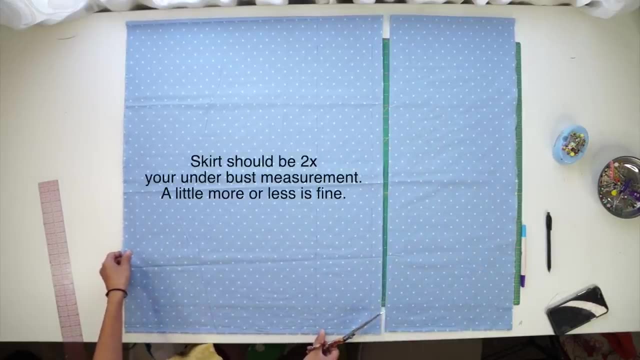 Mark that measurement straight across your fabric and cut it out. I also want to mention that my fabric is on grain already. The rest of the fabric is going to be used for the skirt, which is already two times the size of my underbust. so it'll give me just enough gathers. 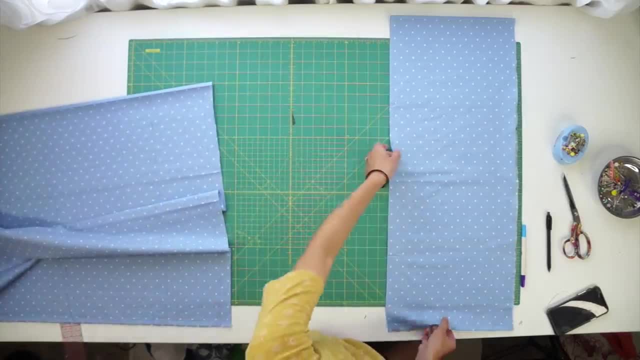 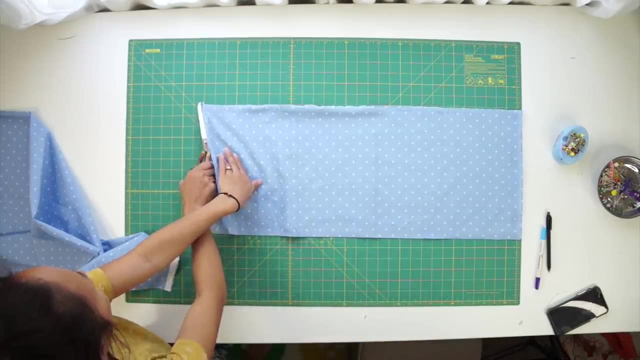 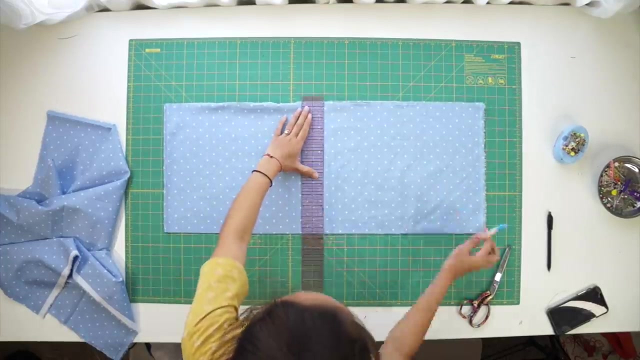 The length is above my knees, but I'm probably going to shorten it later. Next, take the smaller piece, which will be the bodice, and cut open the folded side. Then fold the fabric in half to mark the middle. Next we need to decide how low our neckline is going to be. 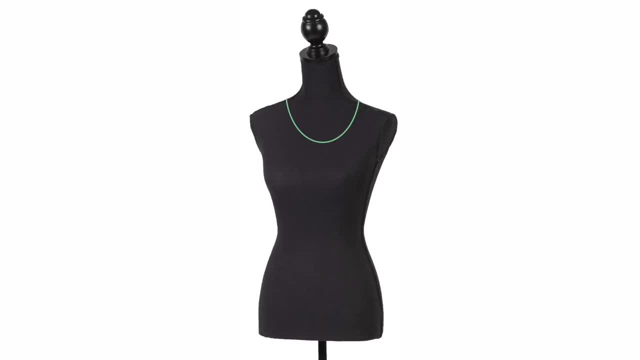 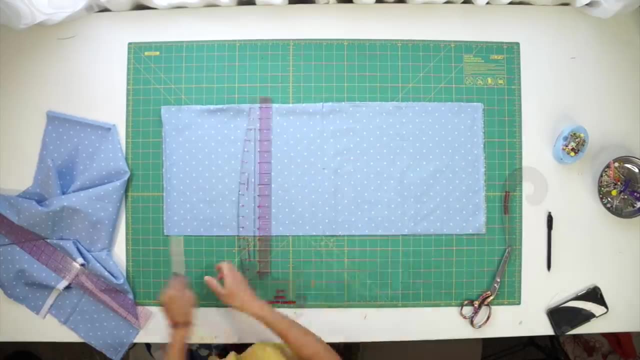 You can trace the shirt you have at home Or measure on yourself to find the lowest point of the neckline. I made mine 6 inches down from the top For the head opening. 7 inches was the perfect size for me, but always measure on yourself first. 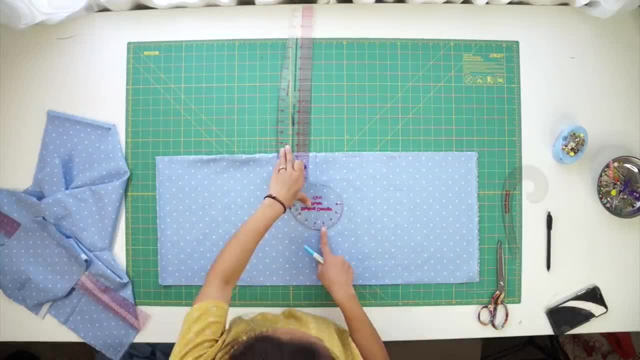 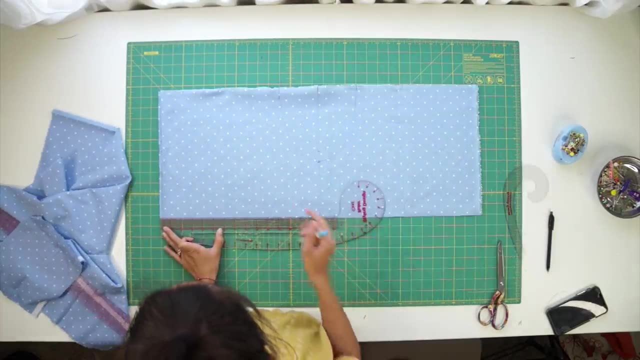 I would even recommend you use a scrap piece of fabric or a piece of paper and cut out the neckline to make sure it can fit over your head. The next markings I made were the underarm seams. Make sure the space in between is wide enough to slide on and off over your shoulders. 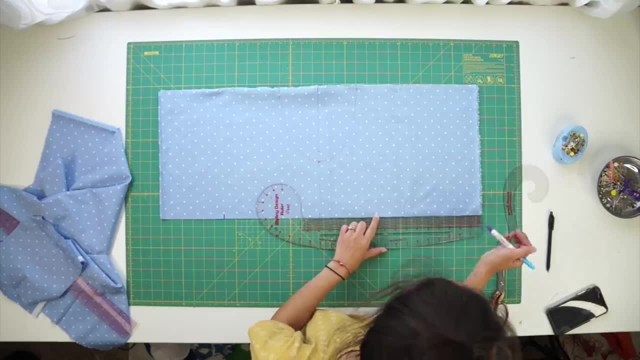 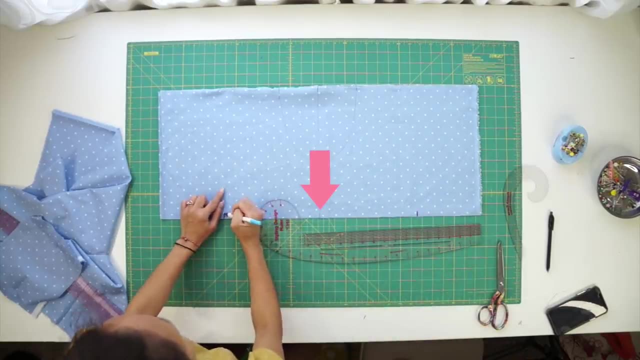 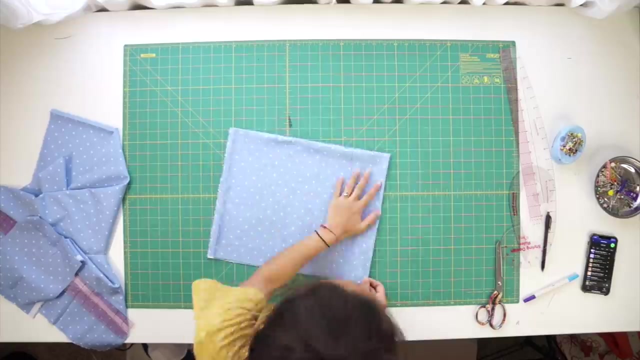 My markings were 5 to 6 inches from the sides. It really depends on how wide your fabric is as well, so just make sure the space in between will fit you. Then whatever is left can be the sleeve or armhole. Once I have those markings down, I fold my fabric in half to cut out the neckline. 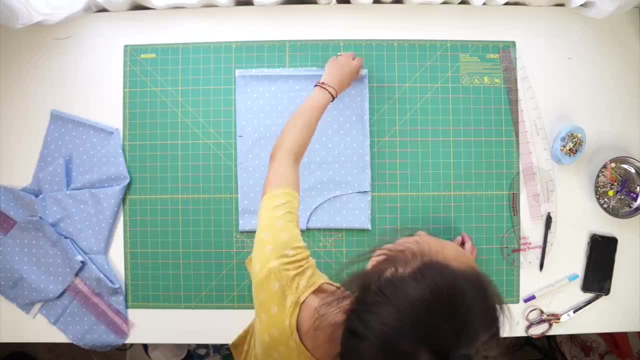 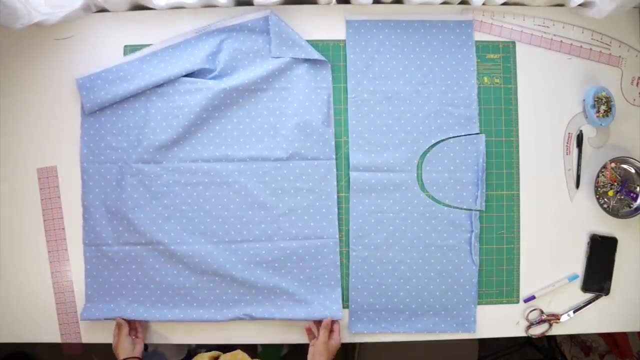 It's important to cut the neckline the same on both sides, because now I can reuse the curved pieces as pockets later. Here are all of my pieces Before I show you how to control the neckline. I'm going to show you how to control the neckline. 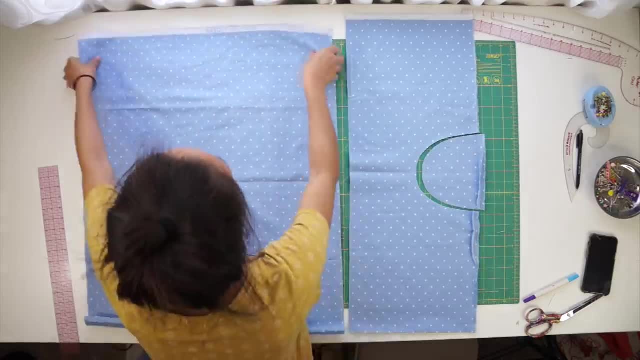 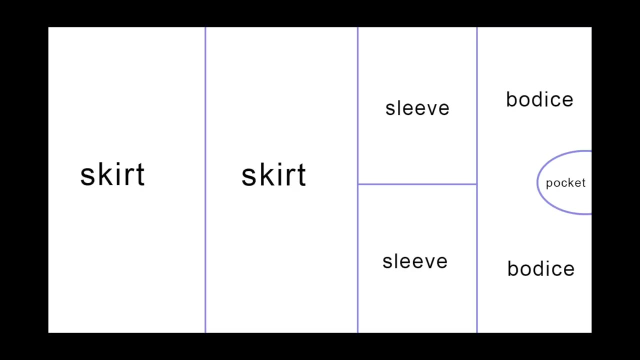 And also how to登録 the dress. Here are some ideas on how I would upsize this zero-waist concept. If you are a bigger size, you are going to need to purchase more than 1 yard of fabric. Lets say this is 2 yards of fabric. 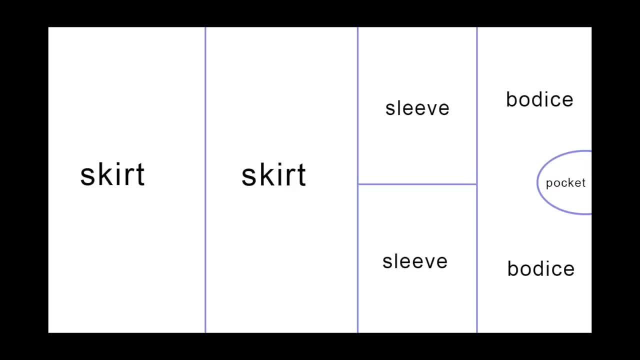 The skirt needs to be two times the size of your underbust. So if you need more fabric, you can cut out two skirt pieces and attach them together to fit you. If the bodice isn't wide enough for sleeves, you can always cut two additional rectangles. 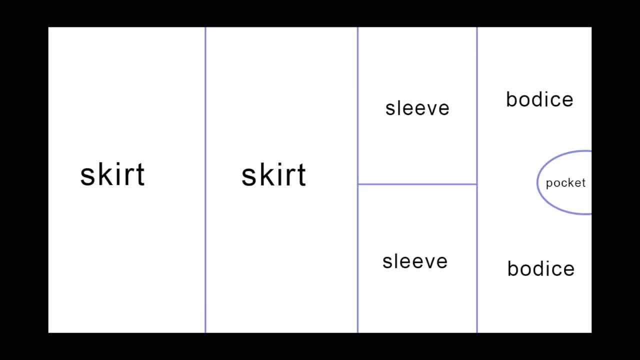 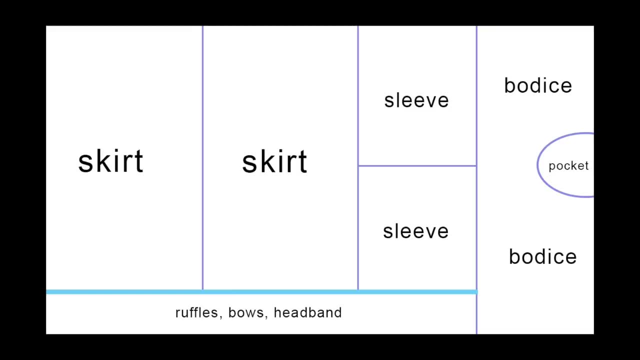 to add on to the sides of the bodice. Now, let's say you're in between sizes, so you'll have extra pieces left over. You could use those pieces to create some ruffles, bows, headband or whatever you can. 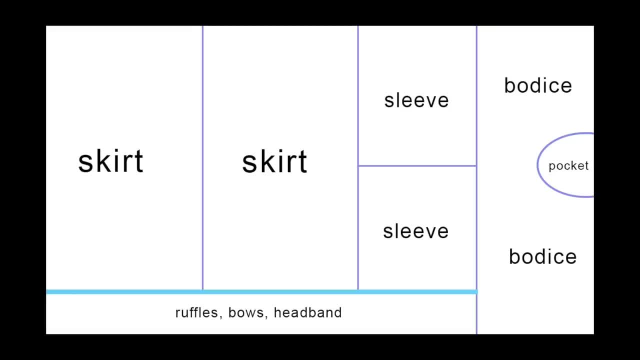 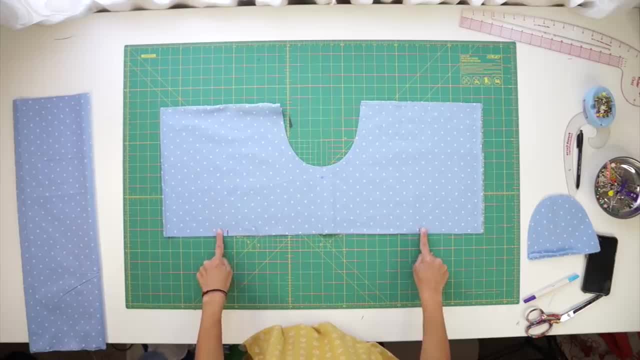 think of. These are just some ideas I came up with, but I'm curious to see how you'll create zero waste with what you have To construct the baby doll dress. first, sew the top of the bodice and the underarm seams. 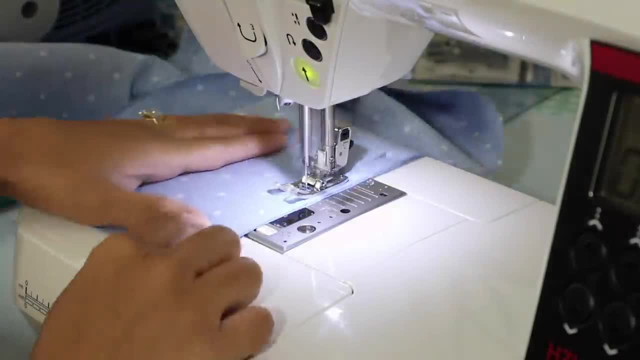 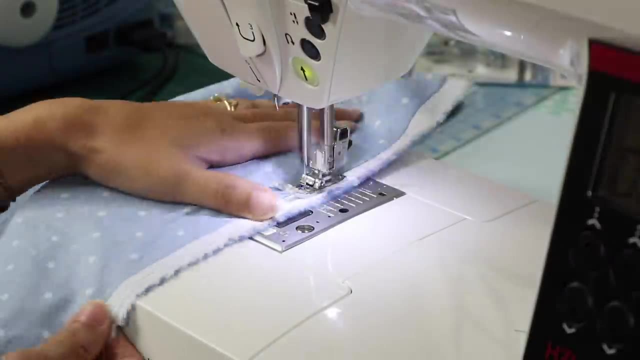 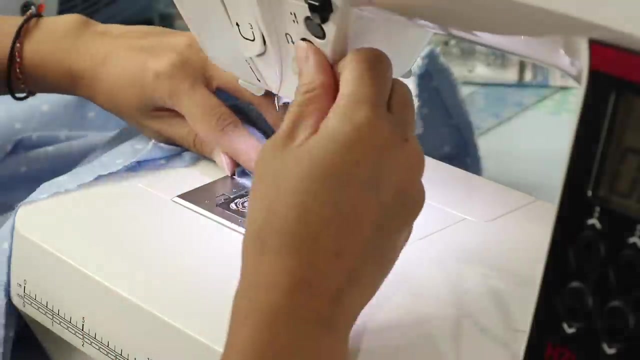 Next, take the skirt piece and sew the open side closed. The nice thing about leaving the selvage is that the fabric won't unravel, so you don't have to finish the edges. Then gather the top of the skirt by sewing a basting stitch and pulling on the thread. 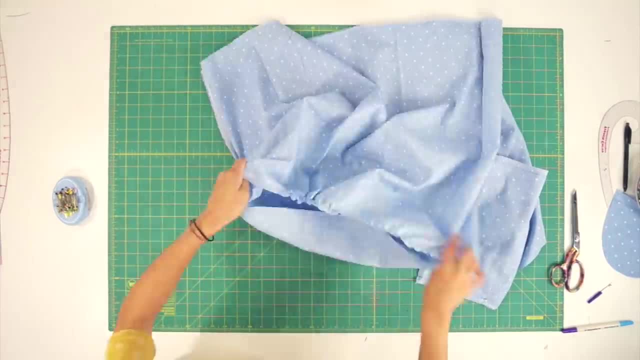 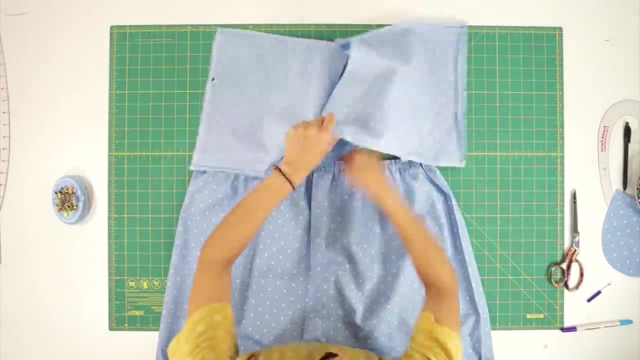 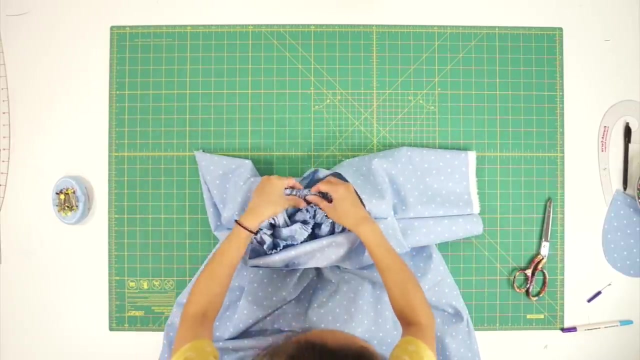 Evenly gather it to fit the bodice, then sew the two pieces right sides together. Okay, The underarm seam I created is kinda awkward to sew because it's straight. so just do your best to pin the skirt right sides together. but if you want to, you can create a little. 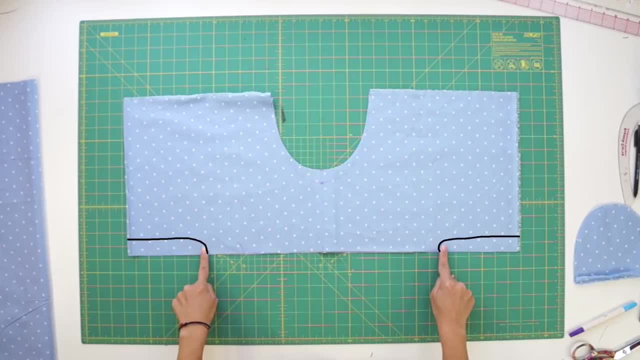 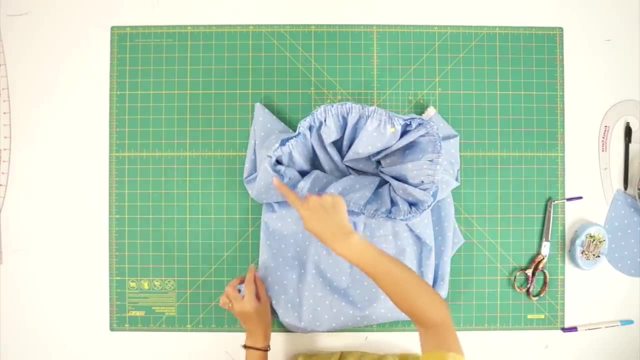 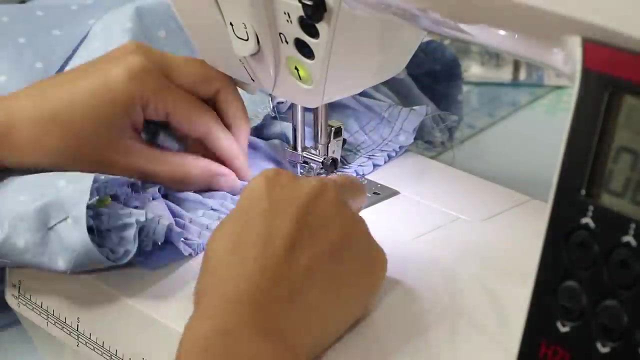 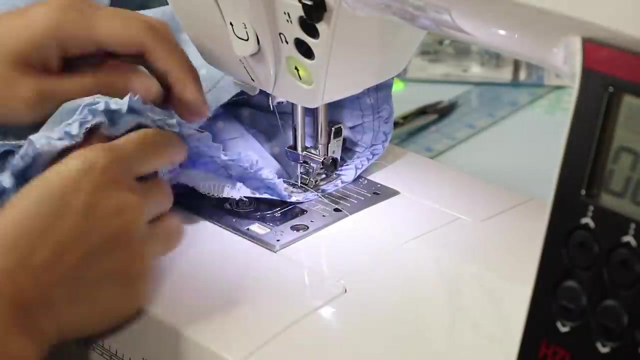 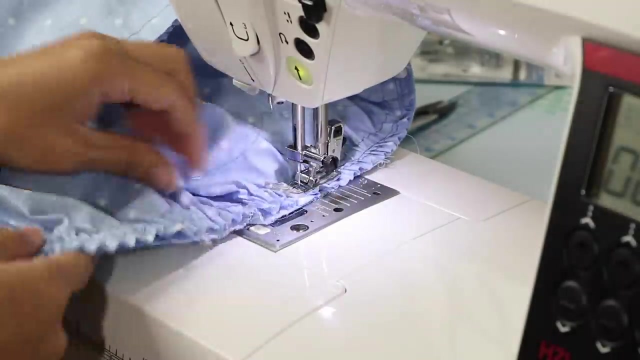 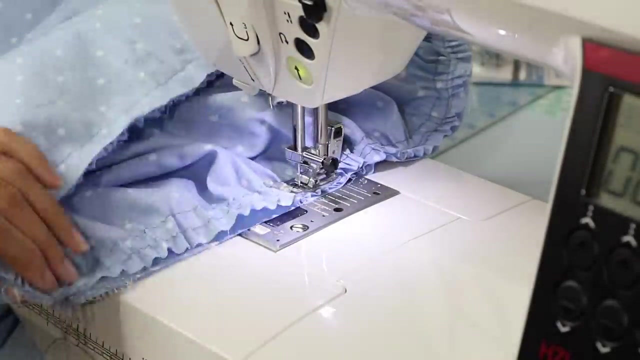 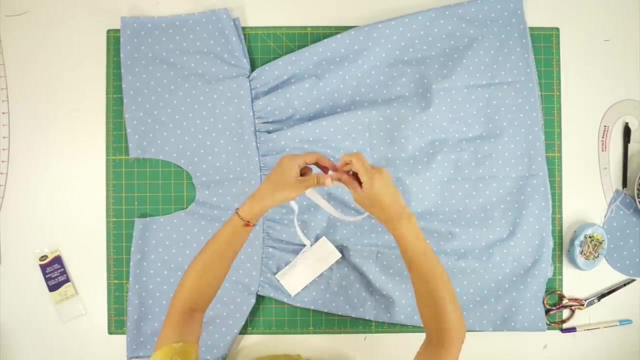 curved shape so the skirt can have something to pin to. I was just committed to this being zero waste, so I avoided cutting anything away. I'm going to sew the bottom of the skirt and then the top of the bodice, Moving on to the neckline. to finish the raw edges, I sewed on some single fold bias tape. 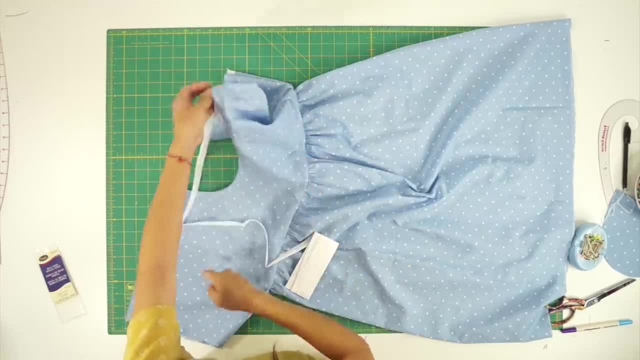 I'm going to sew the bottom of the skirt and then the top of the bodice. Then I'm going to sew the collar on And sew the finished hem. To sew it on, you want to pin and fit the bias tape to the neckline first and sew the 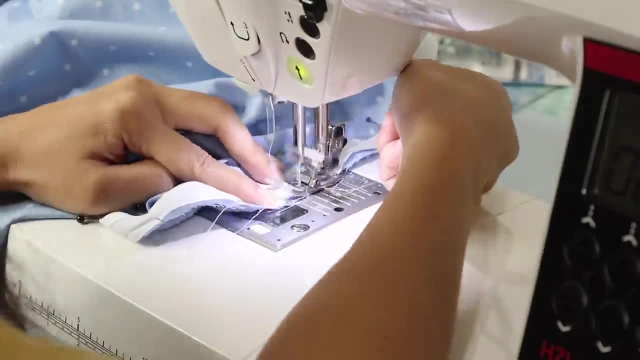 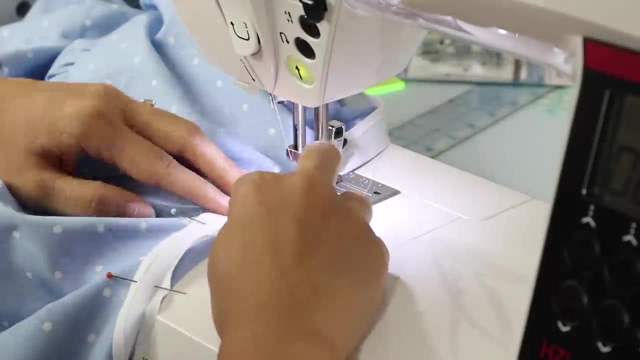 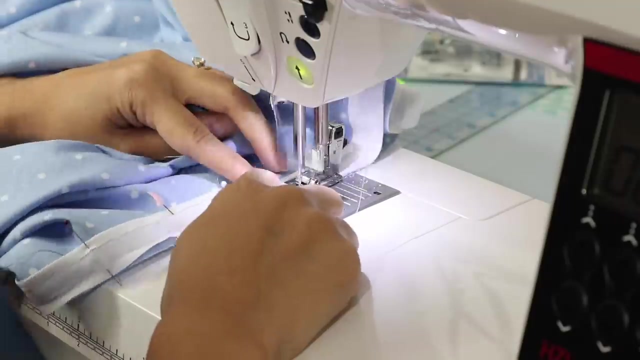 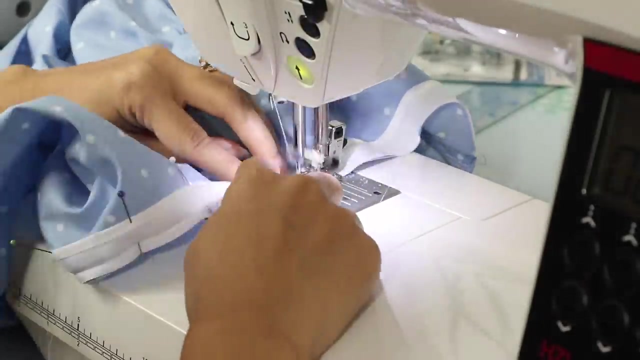 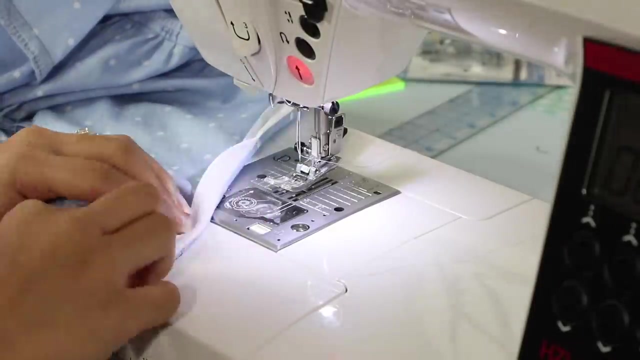 ends together. Then, with the bias tape unfolded, sew one edge right sides together to the neckline. Okay, Done, Looks good. Yeah, Just finished. After that, flip the bodice tape over to the wrong side of the bodice and topstitch the 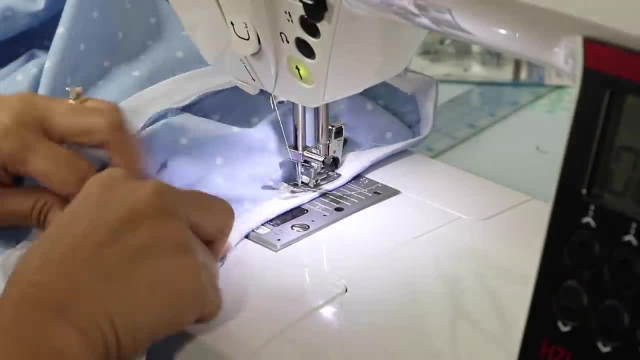 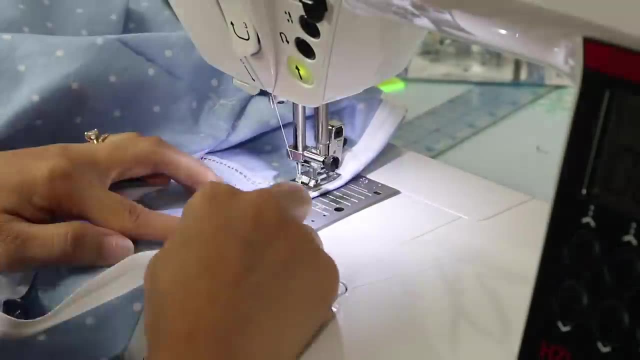 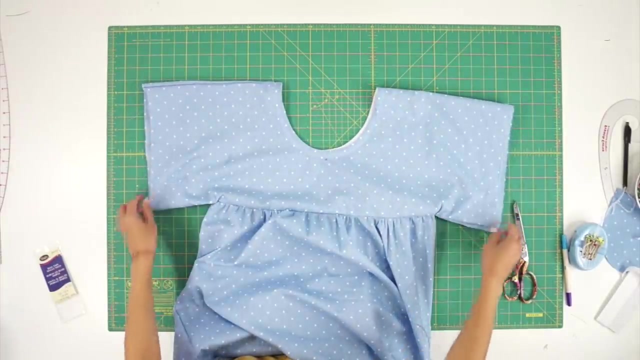 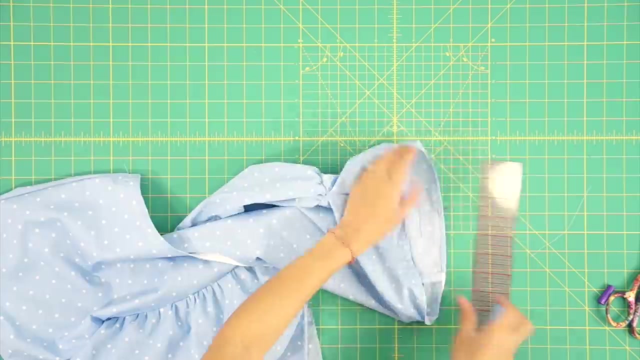 other side down along the folded edge. Make sure to press with an iron afterwards so everything can lay nice and flat And now you have a nice, clean neckline. To finish the sleeves: I first hemmed the raw edges, Then I marked a 1 1⁄4 inch line along the bottom of the sleeves and will be stretching. 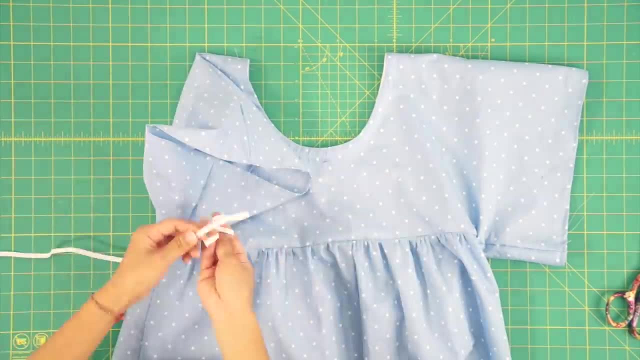 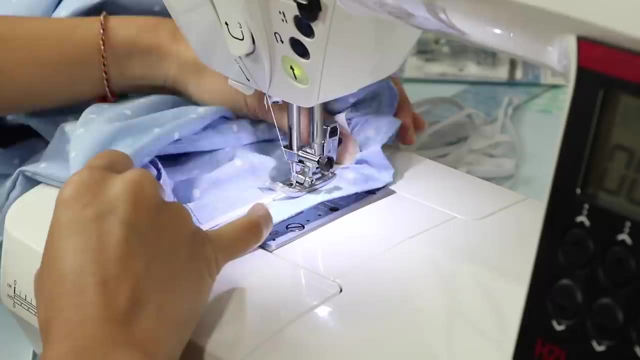 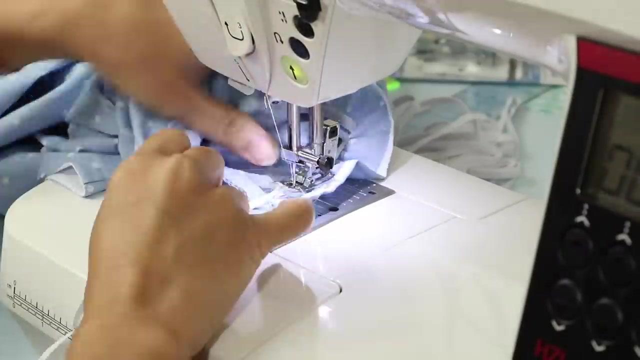 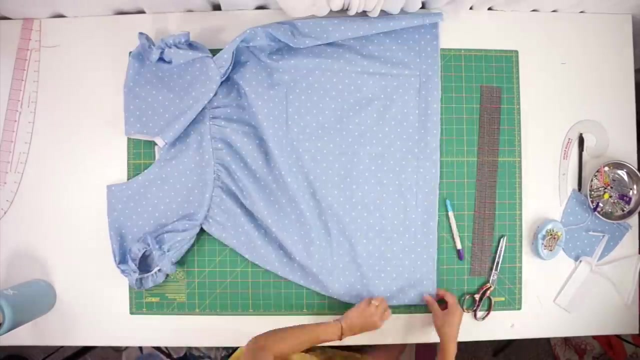 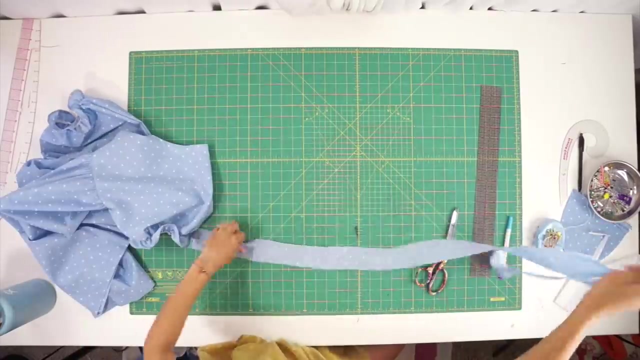 and sewing elastic to create some ruffles and a poof sleeve look. I decided I wanted the length, just the length of the bodice. It's a little shorter so I trimmed off a couple inches and will be reusing it to create a tie for the back of the dress, to cinch it in if needed. 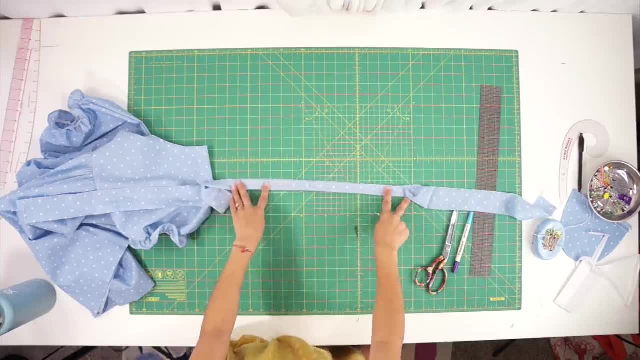 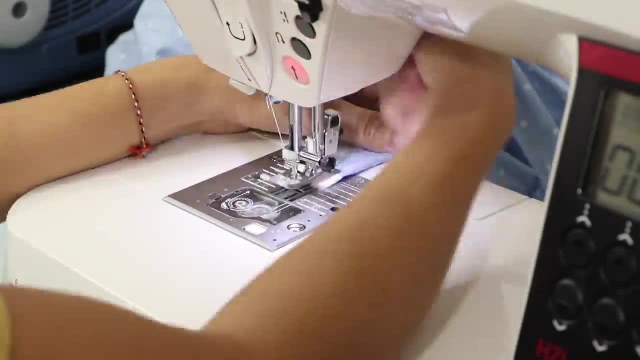 Just fold the strip in half and sew the open side closed. You can make your tie as wide as you want, but don't make it too narrow, because then you'll have to trim some extra material away or you won't be able to turn it inside out. 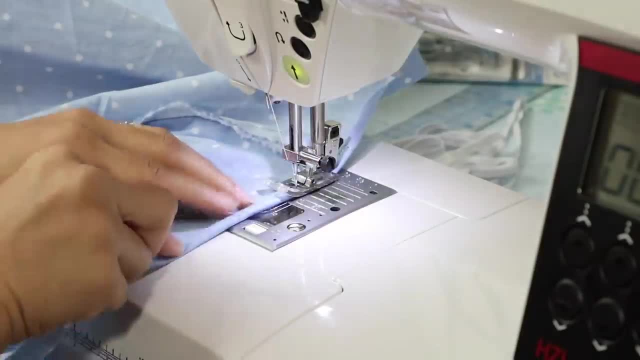 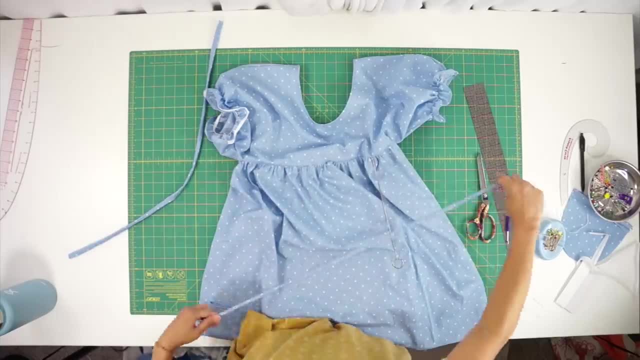 I'm going to use a 1 1⁄4 inch long piece of fabric. I'm going to use a 1 1⁄4 inch long piece of fabric. Turn the strap inside out with a loop turner and tack it down at the sides of the dress. 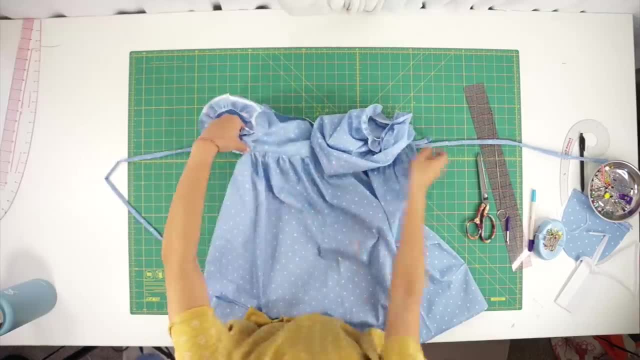 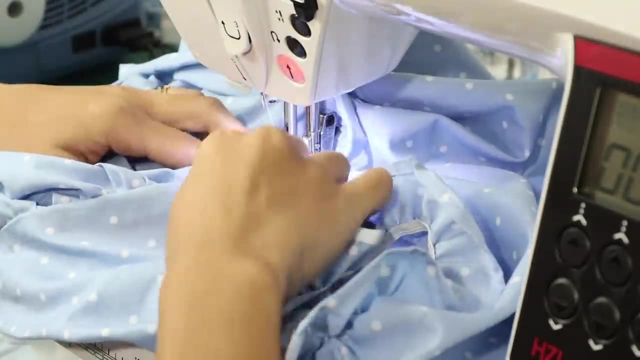 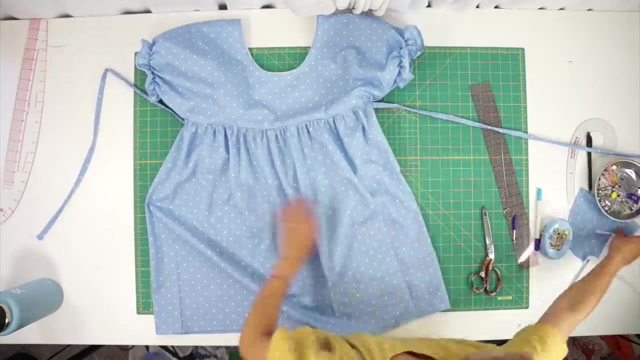 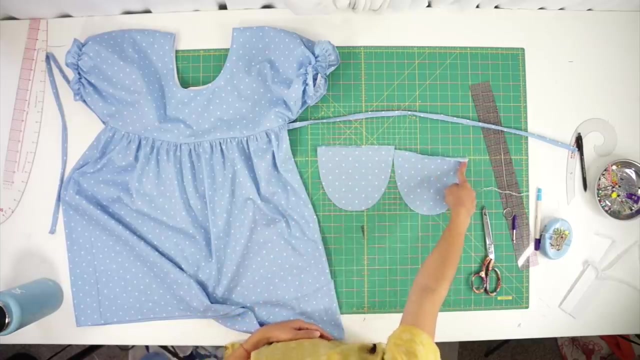 at the waist seam. Lastly, we're going to make the pockets by reusing the pieces cut out from the neckline: First hem, the top edge of the pockets. Then I sewed a basing stitch along the curve and tugged on the thread a little to make. 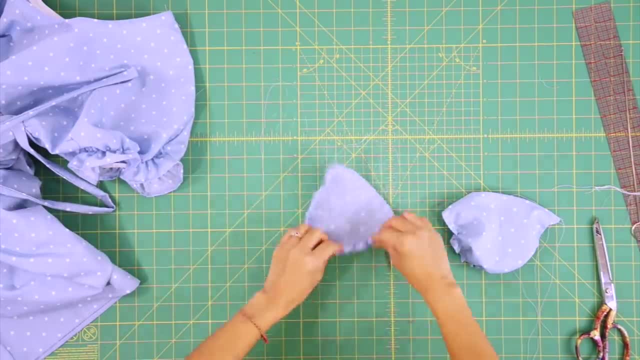 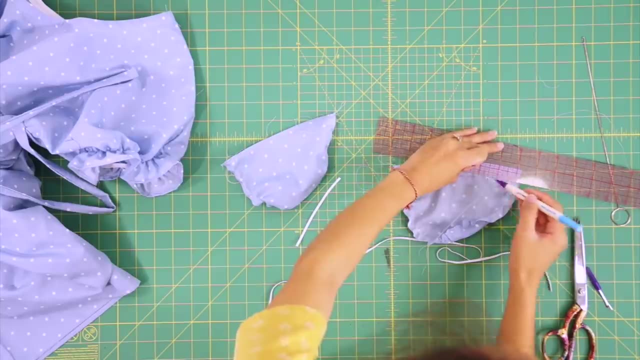 it easier to press the seam allowance in. Then I sewed a basing stitch along the curve and tugged on the thread a little to make it easier to press the seam allowance in. Since the top of the pocket is kind of wide, I stretched and sewed elastic 3 quarters. 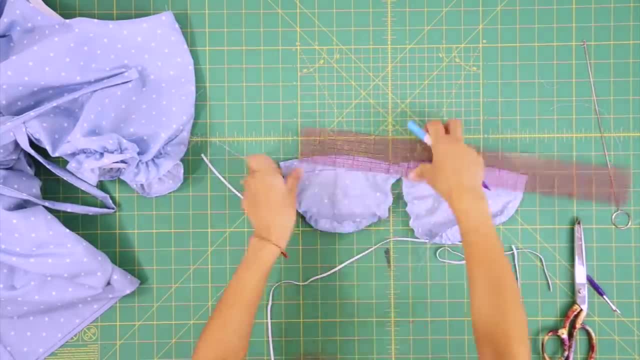 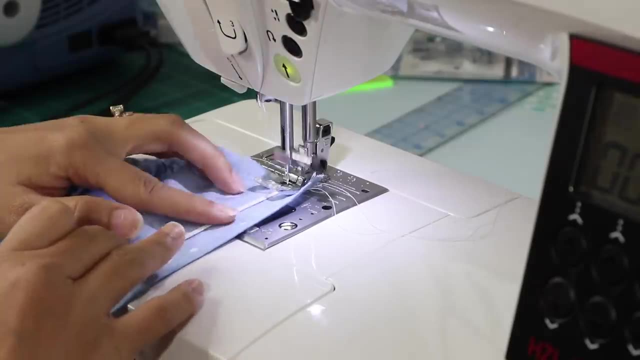 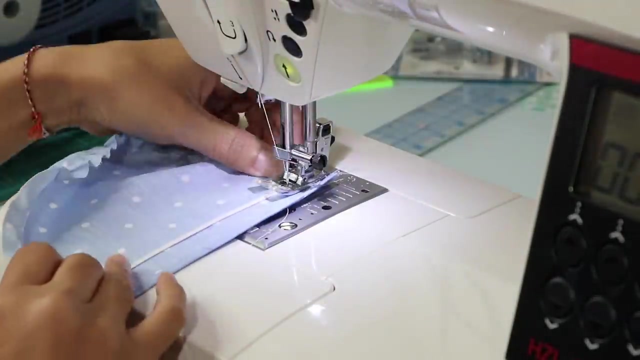 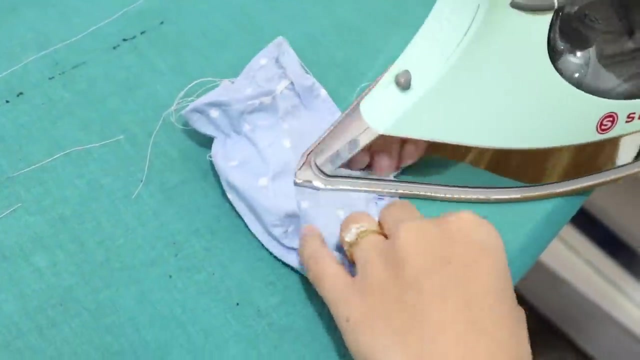 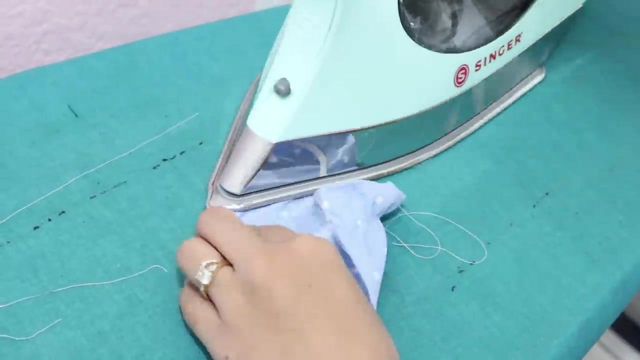 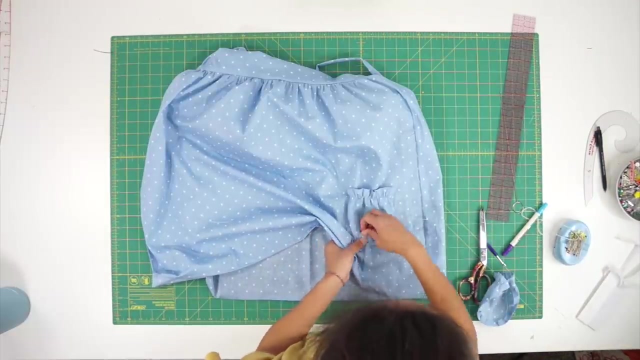 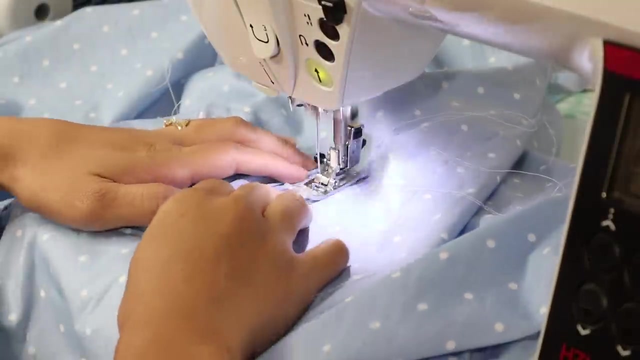 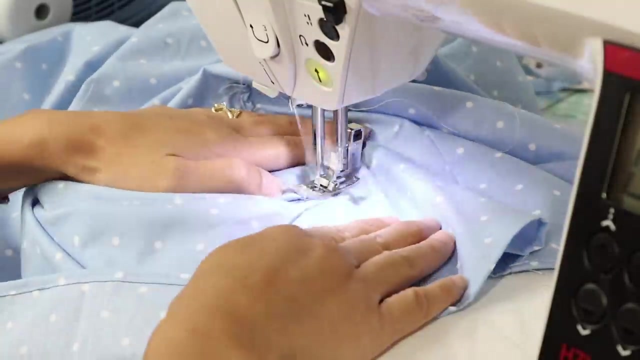 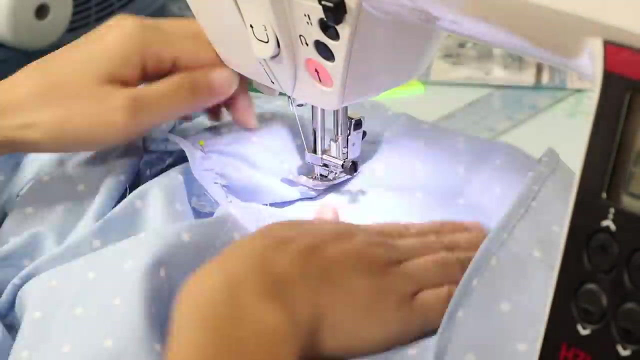 of an inch from the top to cinch it in. This is the vest and the neckline. Next, press the raw edges inside with an iron And, lastly, determine where you want the pockets to be placed on the dress and sew them on. 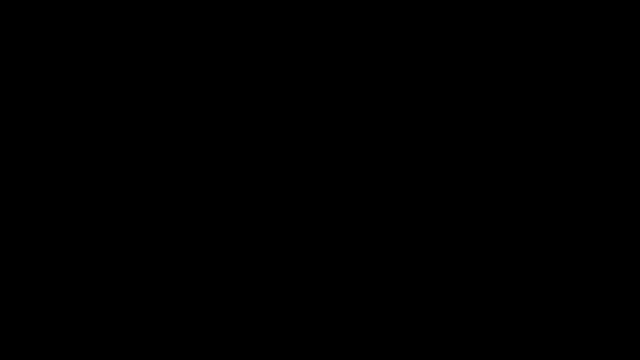 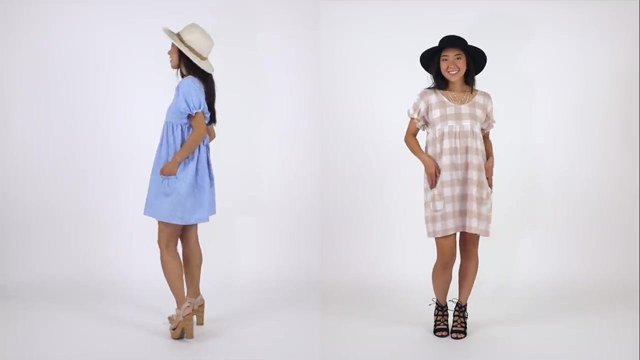 Here is my final creation. I ended up making two because it's so easy and cute, but also because the blue fabric was giving me hospital gown vibes. I don't know if you can tell, but the checkered fabric was not as wide as the blue fabric. 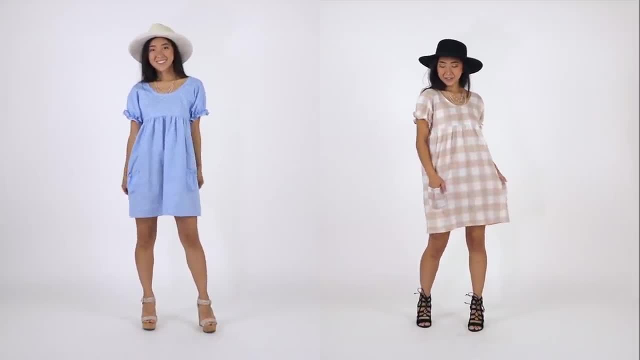 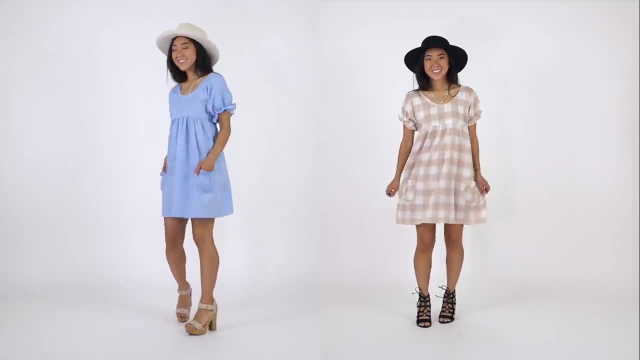 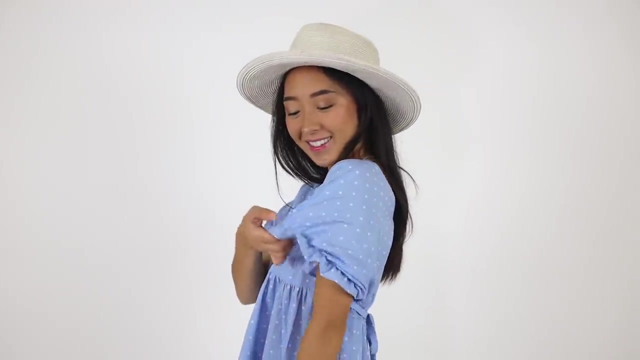 so it has less gathers and smaller sleeves, but it still worked out. You can even make this in a stretch knit fabric if one yard is just a little too small, or add a zipper in the back. It's perfect for a long day's work, since you just sewed the top and bottom in one. 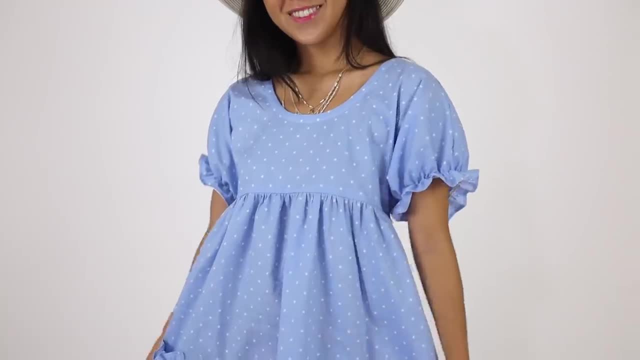 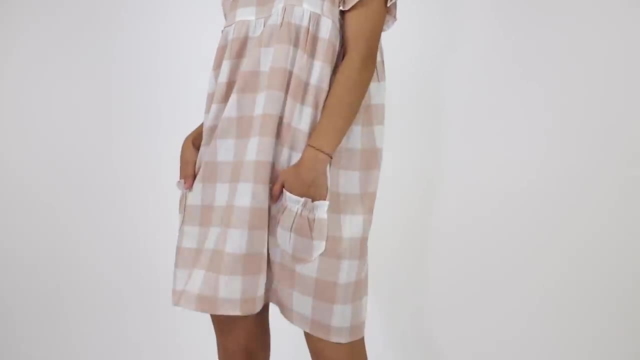 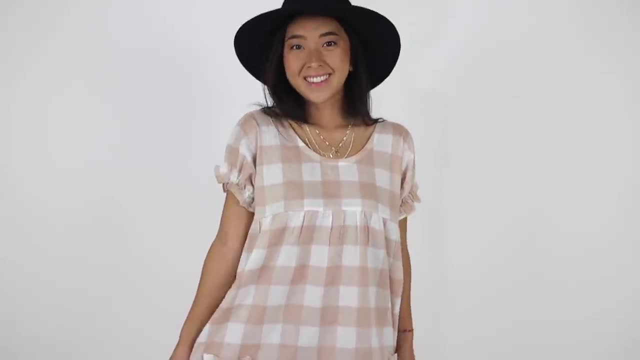 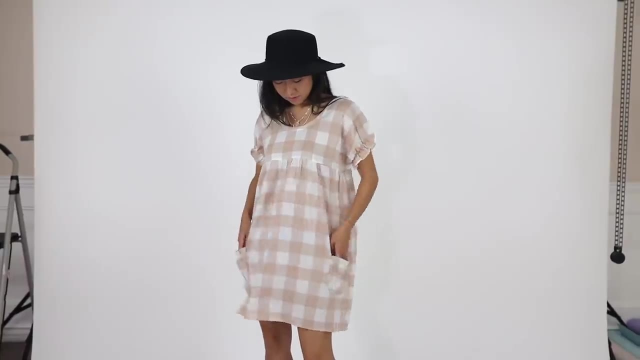 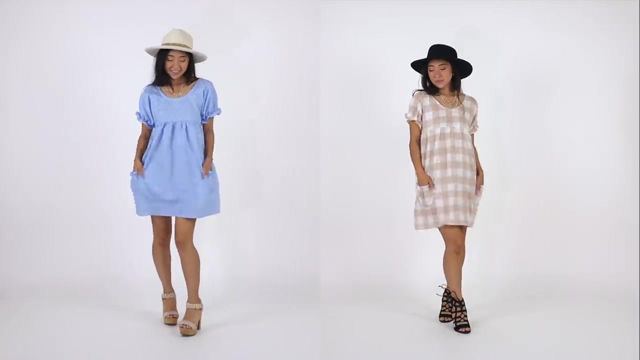 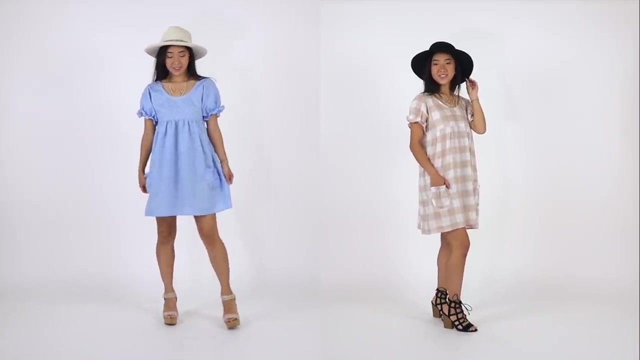